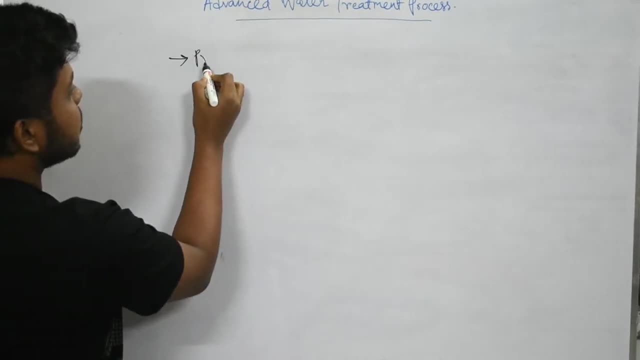 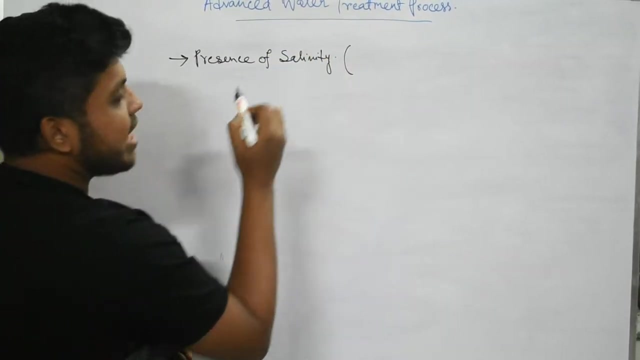 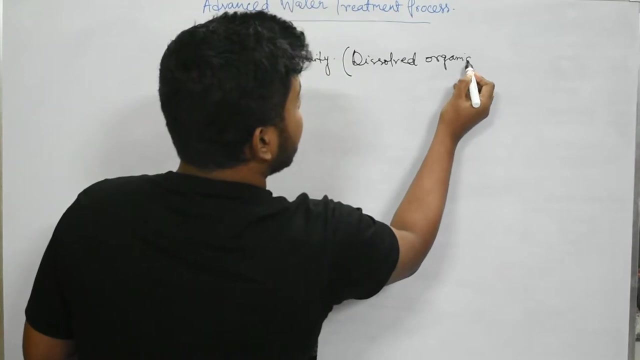 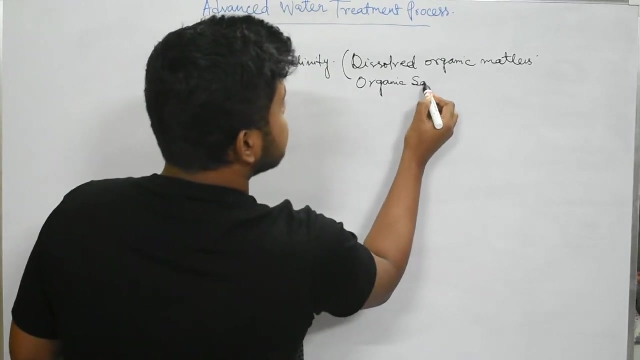 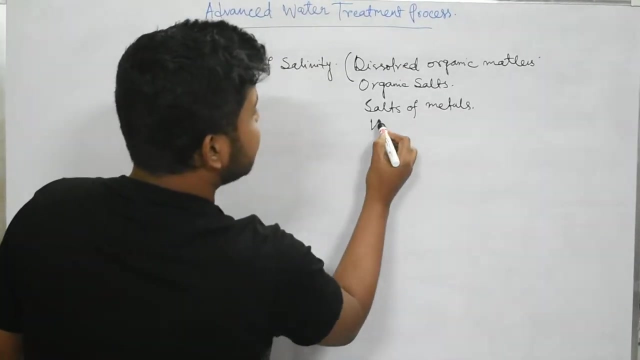 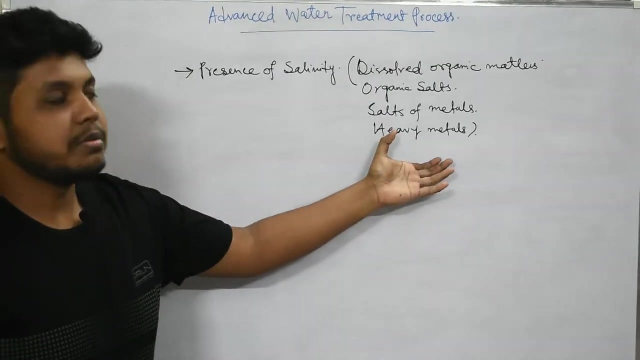 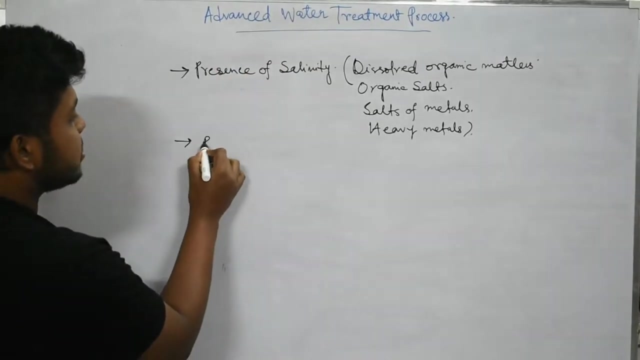 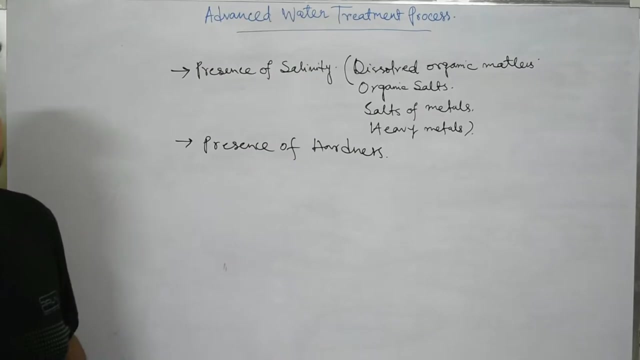 so the limitations are: firstly, presence of salinity. now salinity means the dissolved organic matters, organic salts, salts of metals, heavy metals, etc. these are some salinity causing substances which will be treated by this advanced water treatment. secondly, the presence of hardness. hardness can be overcome by this advanced water. 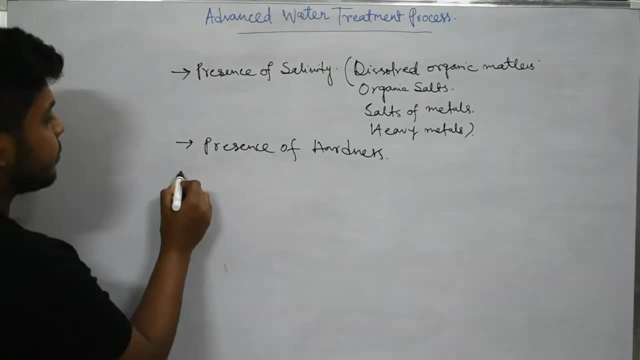 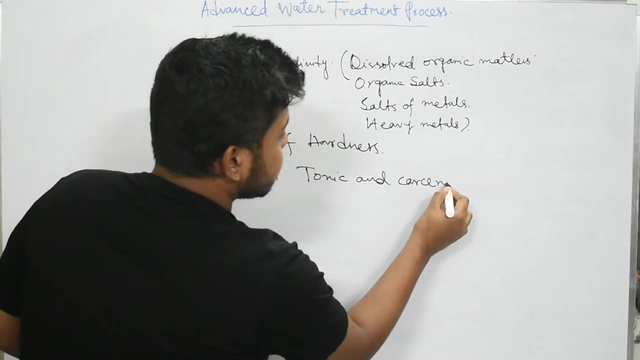 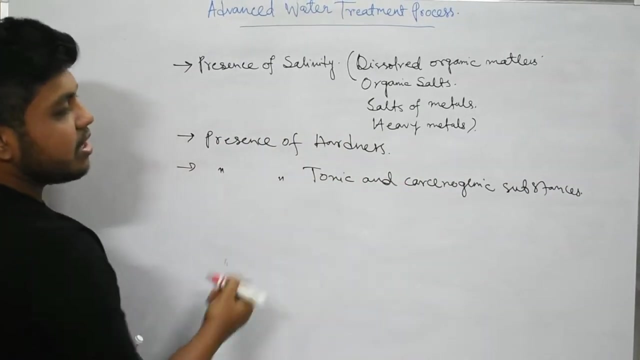 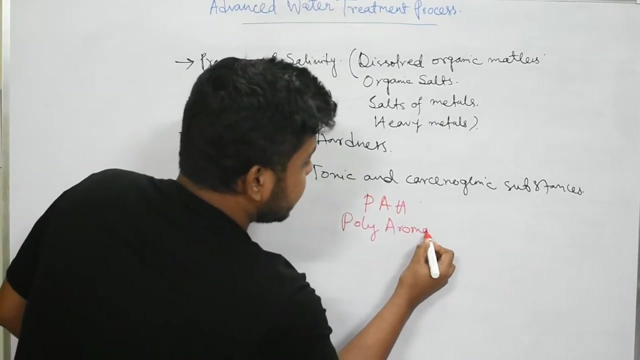 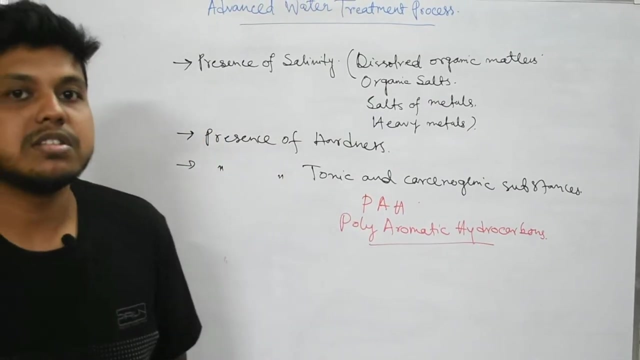 treatment process. we'll further discuss in detail. thirdly, presence of toxic and carcinogenic substances. now, this toxic and carcinogenic substances like p h, that is, polyaromatic hydrocarbons, these polyaromatic hydrocarbons can be get from that polygon industries, pharma industries. 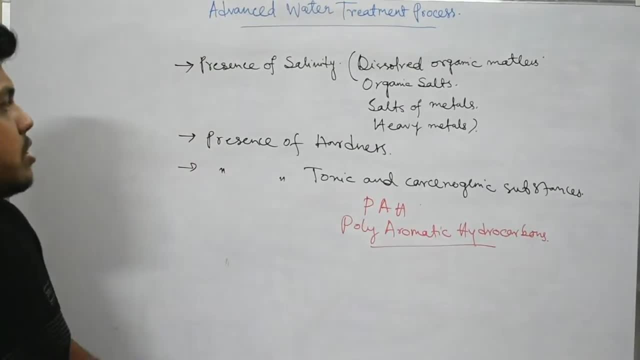 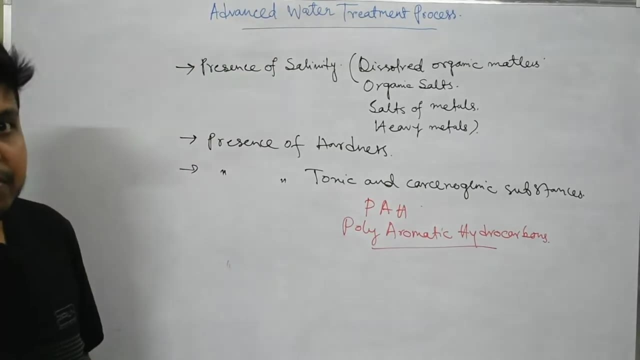 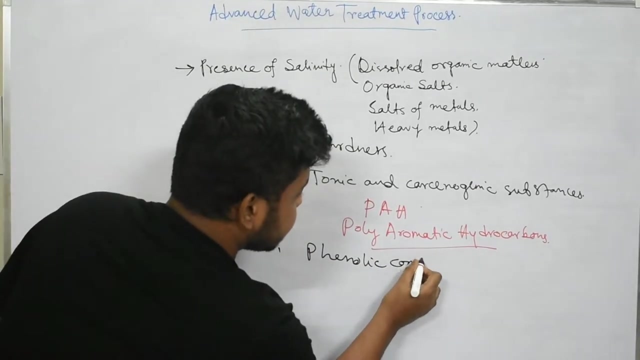 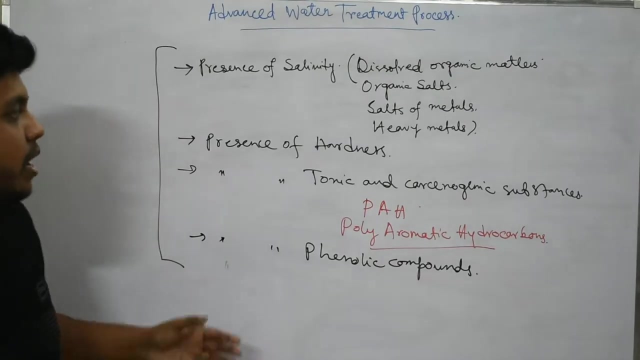 textile industries. so this can cause some toxic and carcinogenic effect if it consumes. so this can be cured by this advanced water treatment process. and lastly, presence of phenolic compounds. so these things are the limitations of that conventional treatment system. this can be cured by this treatment process, so we 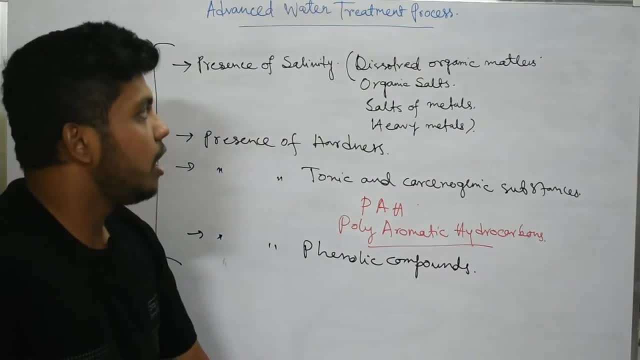 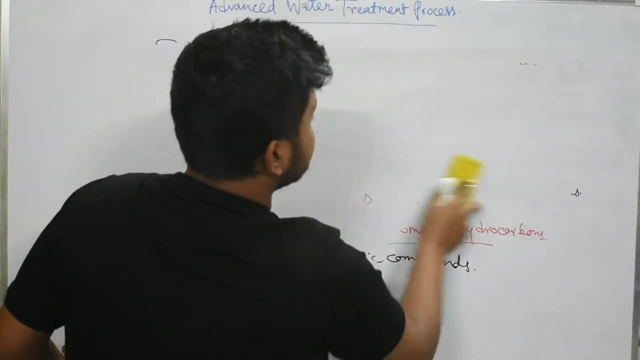 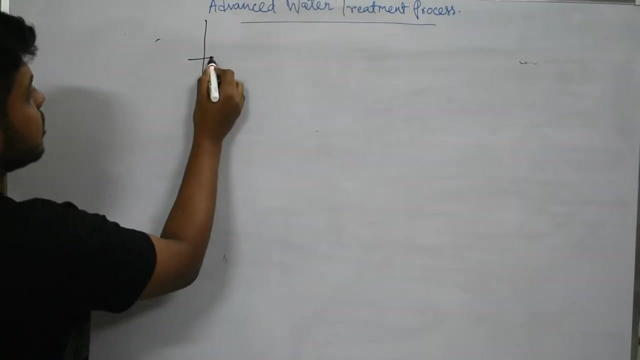 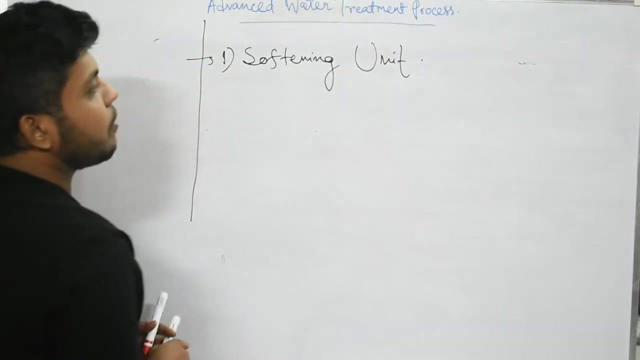 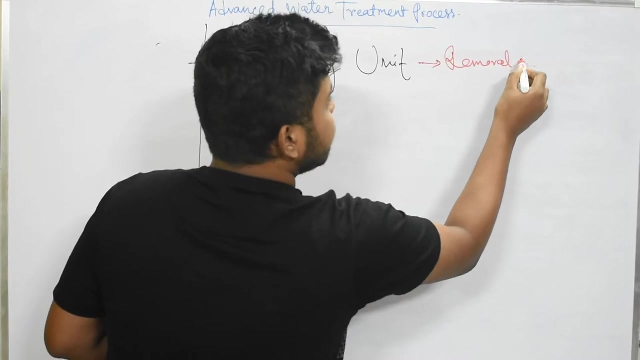 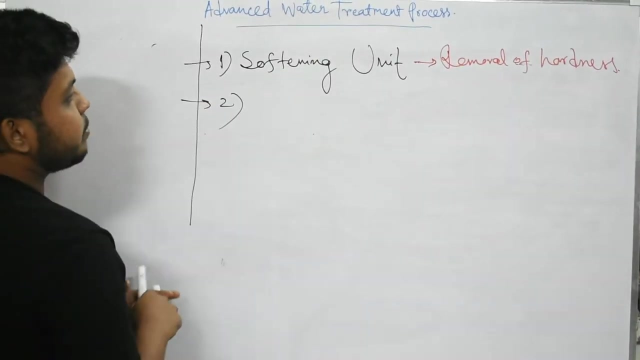 just need to check what are the treatment process we can deal with. so the advanced treatment system are like. so the advanced water treatment processes are number one softening unit. so this softening unit is used for removal of, of, removal of hardness in water. now the second advanced treatment is